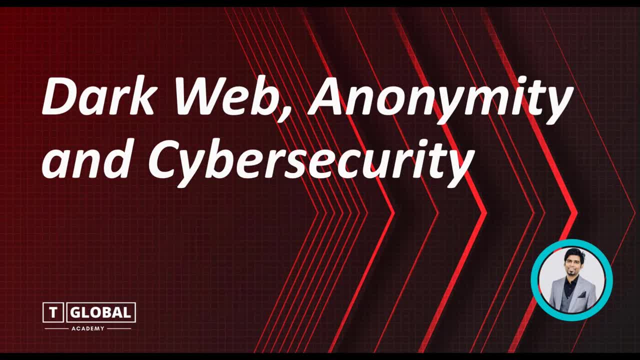 not really the course that we are doing at this moment, but accessing some of the contents that you feel very private. or maybe you are not in a business where free speech is cut. free speeches is really, really important, where your activity belongs to press- alright. so this is where having you having the power of being anonymous is. 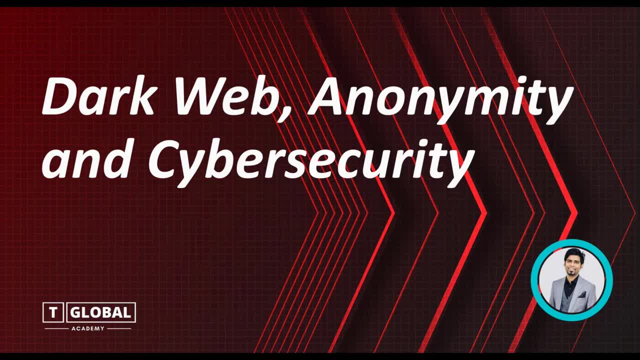 very, very important, and that's where we'll learn more about making use of dark web to access some of to not really to access, but to see what are the different contents available. is it good, is it bad? and for sure it's gonna be bad for 90 percent or 95 percent of the time, but it is important to look at it. what 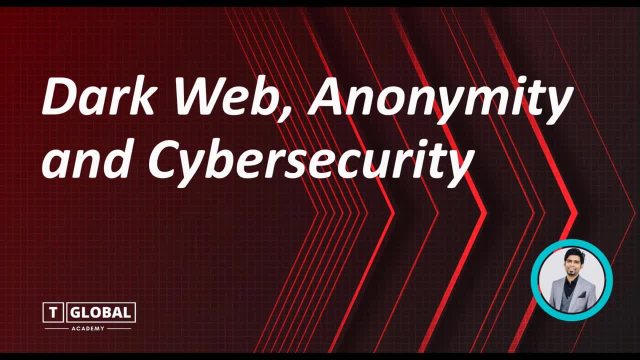 all it is. at the same time, we'll also see if you are even using, making use of your public web, the freely available web. what are the different steps of being being into private mode or anonymous, so that, whatever activity you're doing, you still be safe. alright, so let's get started. 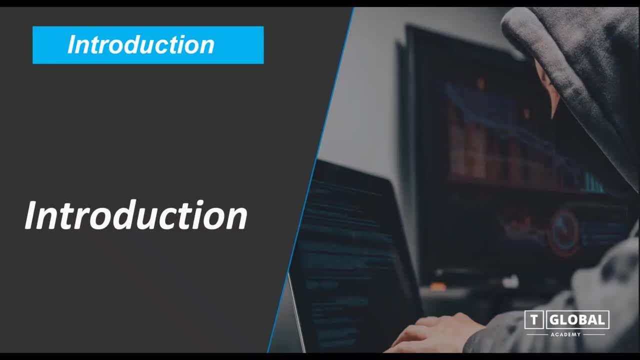 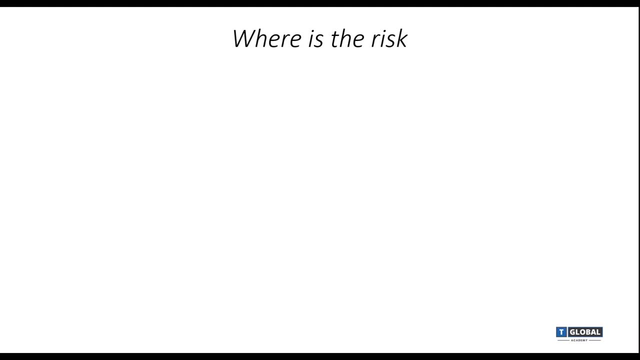 the first thing that we'll learn is the introduction of this course, and over here we'll learn about different risks involved with it. so if you are an user, as I told you in the business of you know those free speech or press related stuff, or maybe in a, you have some content which can send, which can be very 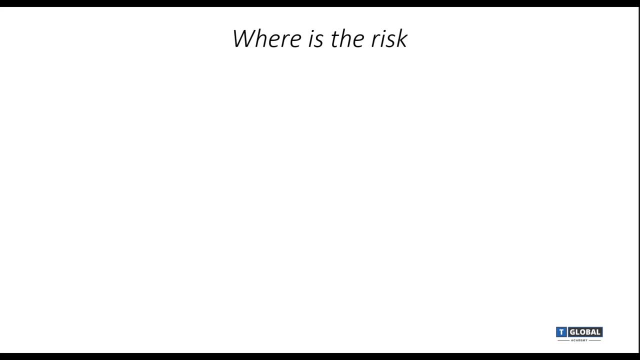 sensitive to some party out there, right? so in that case it is very important for you. but before we get into that, let me just tell you a little bit about the risks involved with it. so before we do that, we need to understand where the risk really resides. all right, the first thing is your hardware itself, your, your system. 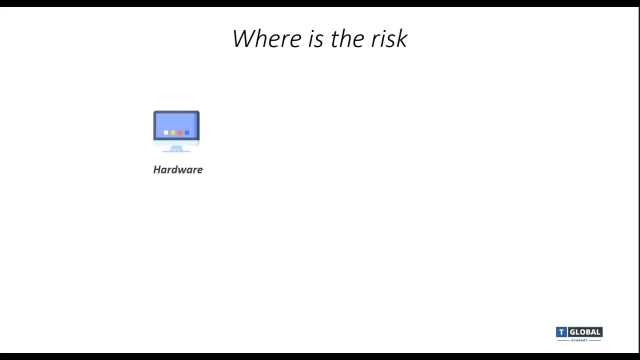 your laptop, your desktop, mobile phone, anything, all right. so anything related to your hardware system from which you're accessing to the rest of the world. that's where the risk reside as well. you might be having your data, but that doesn't get erased, wiped off whenever you you know you you make use. 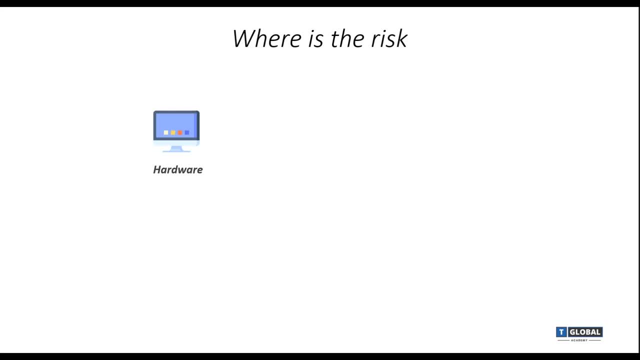 of it. that becomes a risk for you, because that's where the persistence or the part of data that you're using becomes a risk for you, because that's where the persistence or the part of data really resides. even if you're making use of encryption technology, there are 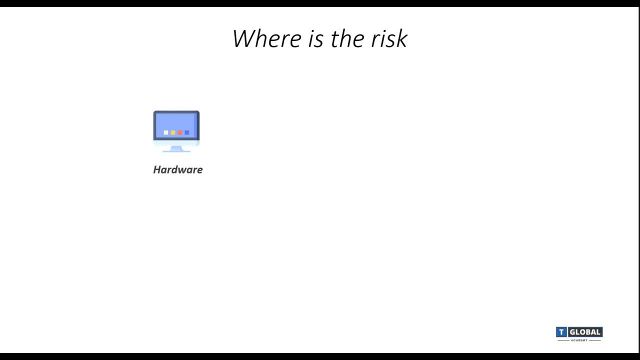 software. there are agencies out there who can grab those information if they, if they want it all right. next is the operating system. now, understand this operating system, help use, help use to make or make use of all your application and that runs on your hardware, right? maybe you talk about. 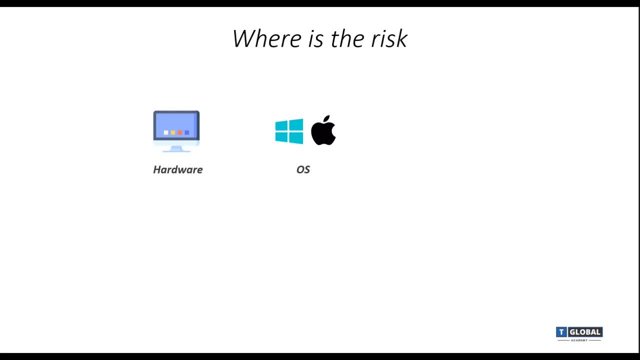 Windows. maybe you talk about your Mac OS. you have Ubuntu, or our clinics, anything, even Kali as well. this all our operating system. and now, if these, these can store the information, because we never know this, the, the open source information, it's good enough, but at the same time, Windows. 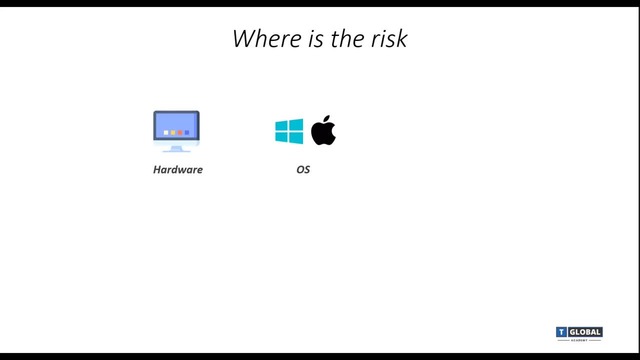 or Mac with these are third party. I mean, this are the private organization and we don't have any control about it, right? so the next thing is the browser. so understand this way: whatever you do in the public network, you can either do it, maybe email conversation, or maybe on the browser itself, and browser is something. 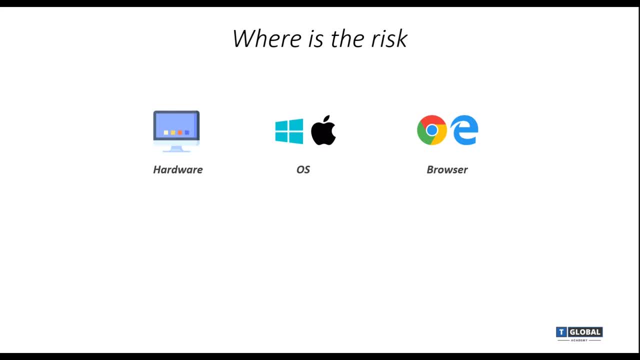 which made all the activity available without installing any agents, right. so, as we are in a situation- we are in the period in era- where everything has gone into the application, starting from your email conversation to chat, to even to your net banking information- or maybe you're browsing. 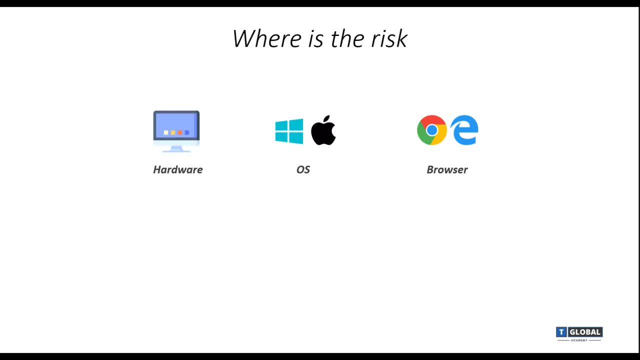 to any effect. everything can be tracked if everything goes to the other party, goes to the any other corner of the world through the gateway and this gateway passes, or send the mirror of the traffic to the national agencies to have a proper surveillance to all their citizen for any purpose, to to influence. 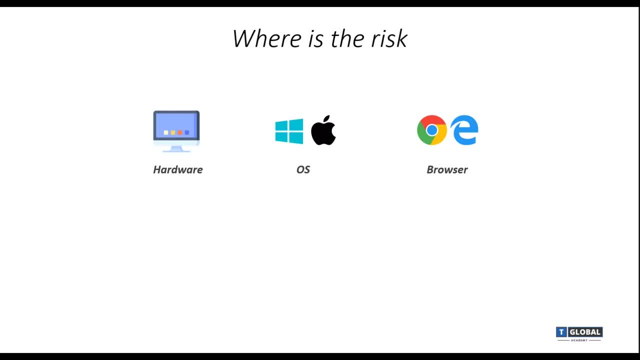 or to have a proper monitoring to their activity. all those stuff, right, and that's where the risk really resides, right. and then it comes to the email. email that you make use of, maybe gmail, outlook, yahoo mail. all these are made for the purpose of productivity, for giving you a useful platform to send an email, but 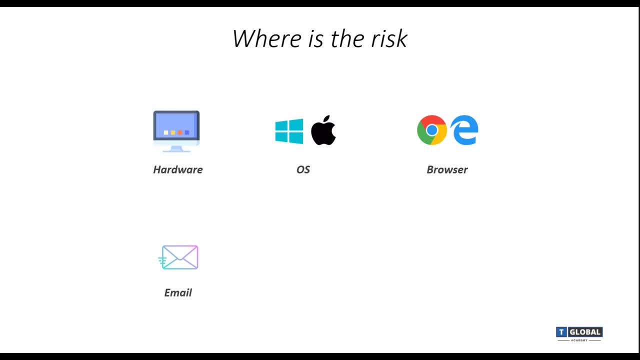 doesn't provide any sort of uh private or anonymity right, because this is where if you send an email, it goes to their server and from there it can be faced to multiple other uh client, or maybe it can be sent to the uh receiver as well. so there's no sort of anonymity, no sort of sort of 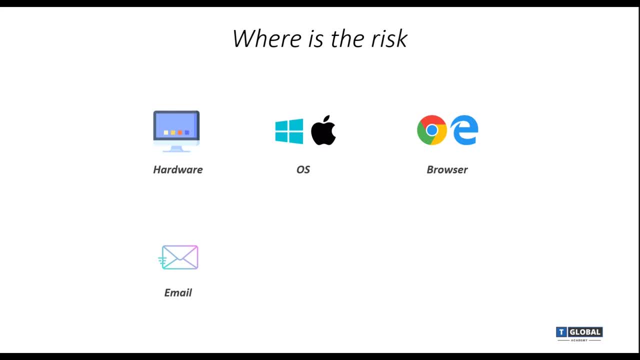 private uh, or making it anonymous as well. the next thing is your wi-fi. now this is, of course, it sounds really crazy, but yes, it is, because if you have, uh- i'm not sure if you have looked at my earlier uh- other ethical hacking content courses- you will find if somebody it's get the access to. 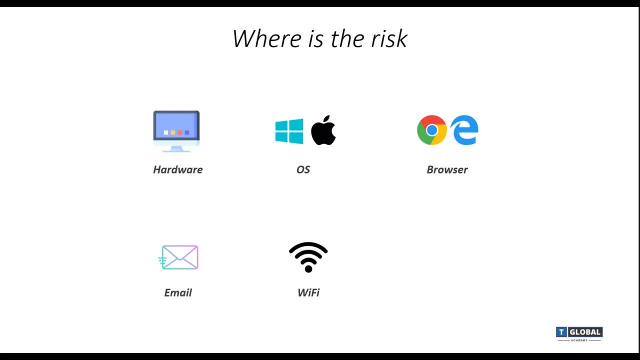 your wire list network it can see. it can actually get to see what all you do, right, with the help of man in the middle attack, they can get to see what all you're doing in your, in your browser, or from your, what all communication going out of your laptop or from your network can be seen or can be, you know, can be. 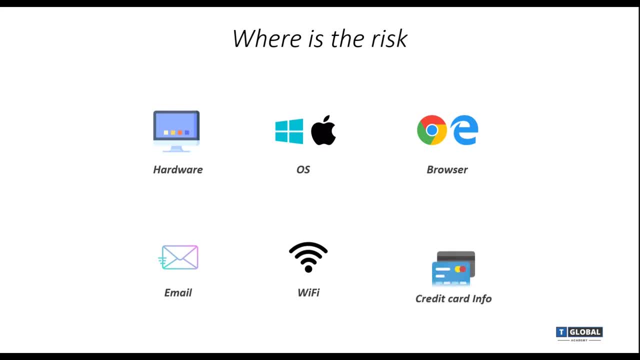 spied as well. somebody can see that personally. all right now at the end. i know it sounds some some sound some very, very different stuff. but yes, of course, credit card information. how exactly? that's a great question to answer this- when somebody share their information as a part of credit. 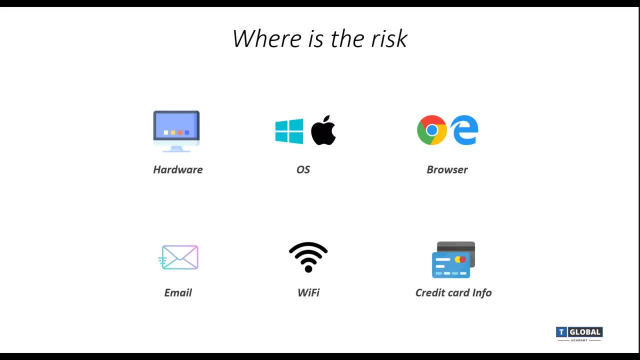 card or maybe any other, any other information, like social, uh, ssn or any other information. anybody can locate them right. because if, even if you're buying something and you're sharing information like your credit card, people can track okay, who, who was the one who bought this information? 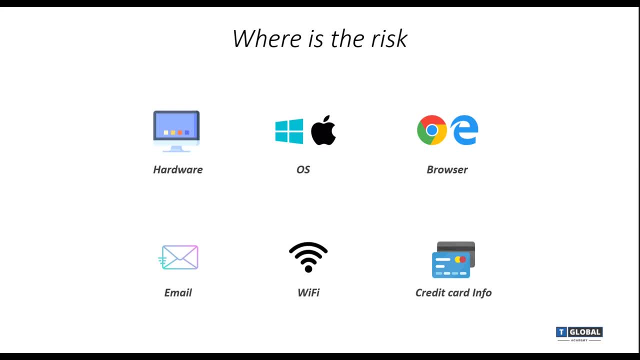 because that's where your name, address and all those information has to be filled up and it can be tracked as well. now, um, it is important to understand how these all risks can be covered at the end. right, and that's that's what we. we are talking about, while being anonymous, being into 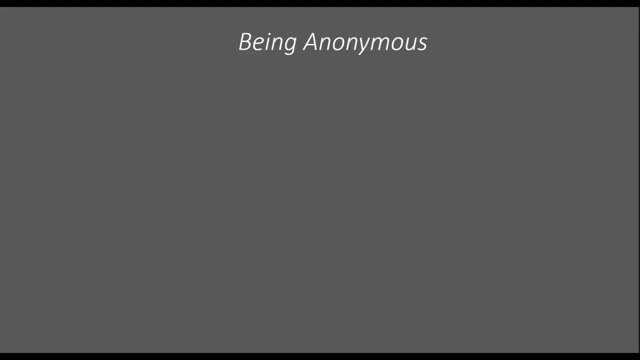 achieving the privacy as well. so this is all about it. now let's talk about how to secure, how to uh reduce the risk, or how to reduce the risk on every layer. so we talk about for our risk at the hardware, operating system, browser, email, all right, so we'll talk about each one of them one by one. so let's first talk about 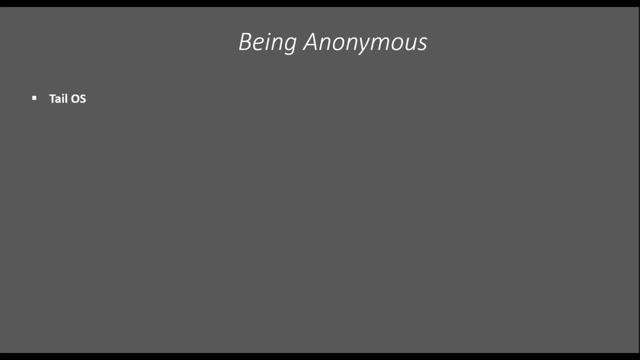 the operating system, and this is where you can make use of telos. what's so special about it? unlike any operating system which has to be binded with your hardware, you know, i mean of course the macbook, your, your mac os can only run on the apple, of course, but for the rest of the 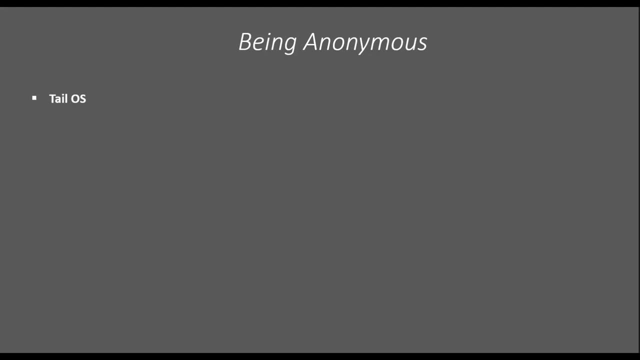 hardware. like you know, the macbook can only run on the apple, of course, but for the rest of the hardware, like hp, dell, windows can be installed or any other operating system can be installed. but remember this: the data still still resides with it once you install any operating system. 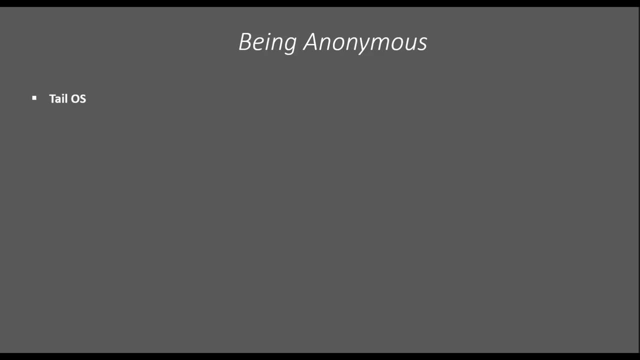 the data resides with it and your operating system can bind those information, can can store those information. and when you make use of telos, it is built to make it non-persistent so you can make use of a usb drive. i'll show you in the next video. so when you make use of telos, i'll show you in the next video. 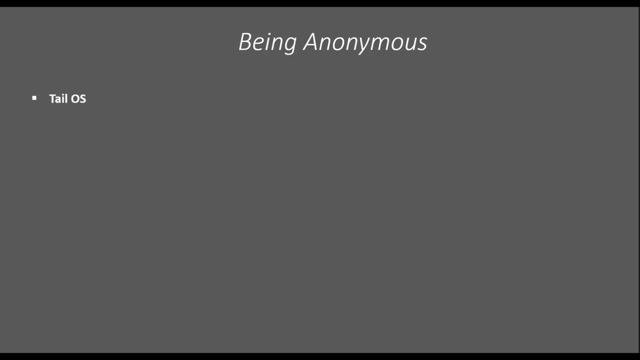 the later courses where you can have a bootable pen drive with telos and this tail. always you can. once you insert, insert on any of the laptop, it just good to go, you can do your work and once you remove it, it wipe up or wipe out all all. 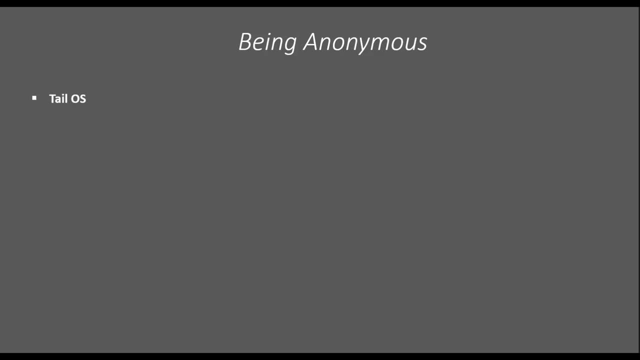 the information, all your activity that you have done on this. but that's useful, all right. next it's it's star browser. we have talked about the risk related to your browsing activity. broad browser is something will be making use of it when we- when we try to access or try to see what all stuff are there on the dark web. 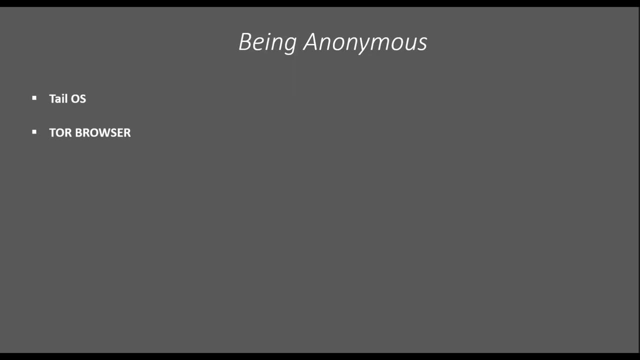 right and this is we are going to learn and we'll see for the educational purpose. why I say that? because this is something which is very, very important. dark web is something which is mostly used for the bad activity and for the educational purpose. wanted to see what all are there in the dark web so that we can educate others. 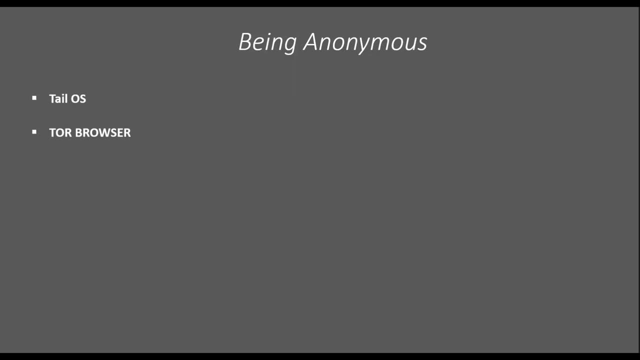 how to make yourself secure and not to go on any dark website- dark web or dark net, you know, just for sake of exploring it- and how to be safe enough before you do any activity over there. all right, so now next hotspot: Wi-Fi: make use of your. 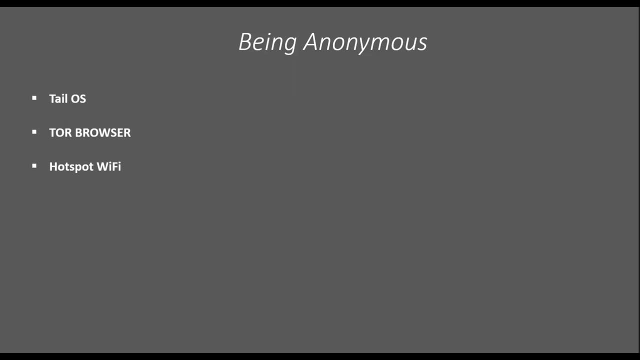 hotspot Wi-Fi whenever you go, wherever you travel. don't make use of any public Wi-Fi activity and, of course, I'm talking about some best practices in the same stuff itself. of course, open PGP, and this is something which is very important. this is a very old technology, but this still works, because this is 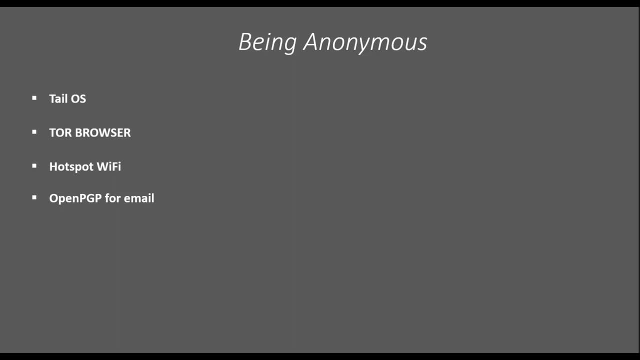 where you know no provider really comes in. you send an email, you get encrypt. you, you encrypt those email content. other party: if he has the key, then only he can decrypt it and can see what is there inside. all right now, this is all about making your email secure enough, or I mean safe. 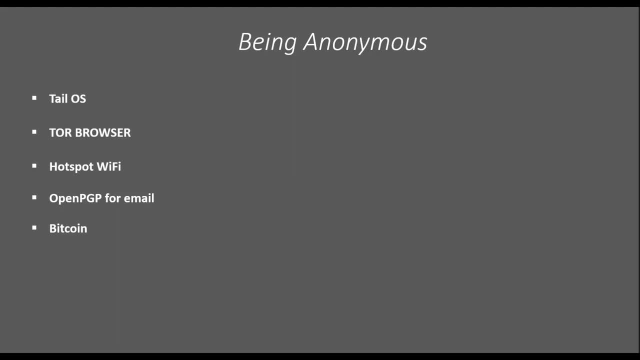 enough, private enough, but coin. I know I don't all of you know Bitcoin right, but we are talking about it for, not for making money out of it, not to have a precision or valuation, all those stuff. but what I'm talking about is if you really want to make yourself anonymous on the on, anywhere in the world, in spite. 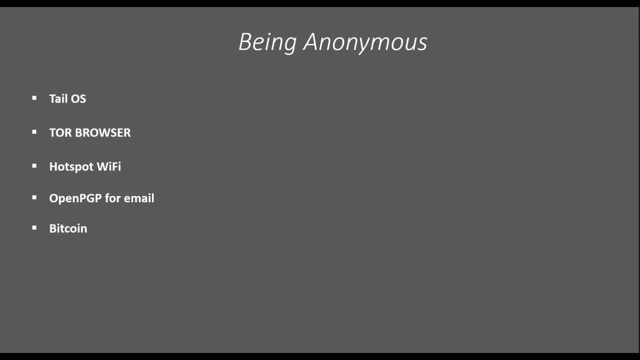 of using your credit card information. make use of Bitcoin, because that's where your personal information never get shared. all right now, burden or personal laptop. if you remember, I talked about the risk related to your hardware, and this is where you can avoid that by making use of any of the non-personal. 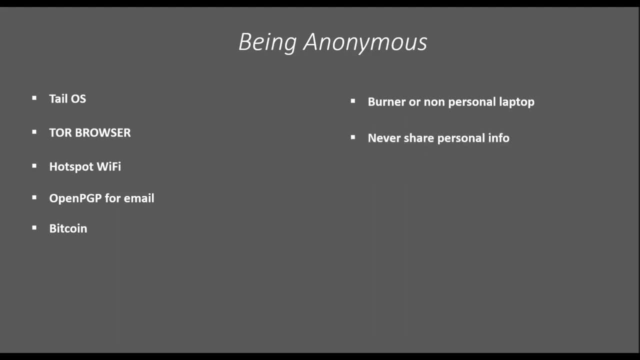 or burner laptop, all right, never, never, ever, never ever share your personal information with anybody, right? because this is where, even if you tried everything, you try to reduce the risk of your personal information, and that's what you're going to get the risk on everywhere if you share your personal. 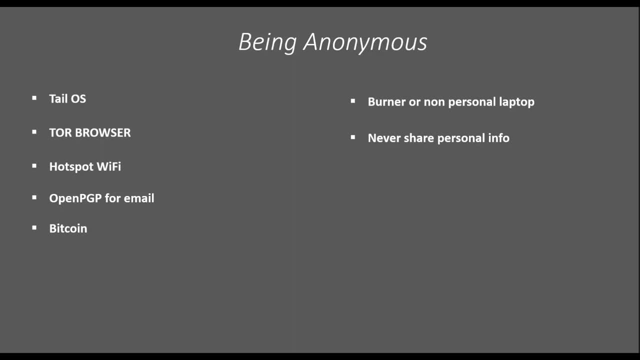 information. there's no, no way to go right, because you never know where it exactly going around right and how it can be used. now, what I'm really talking about at the end is what, whatever we are going to learn, this is all on the personal for the educational purpose. so make sure, make sure you never do any.